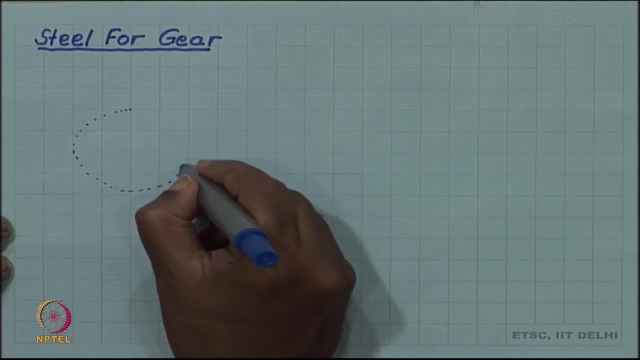 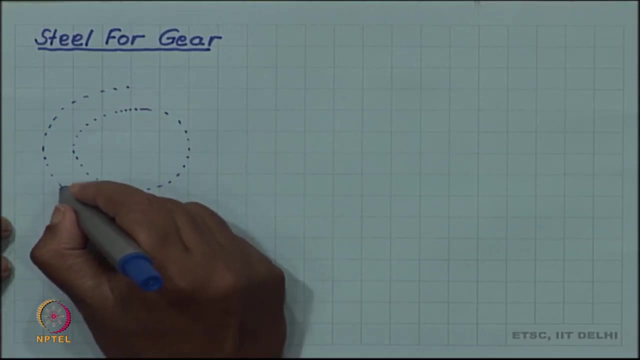 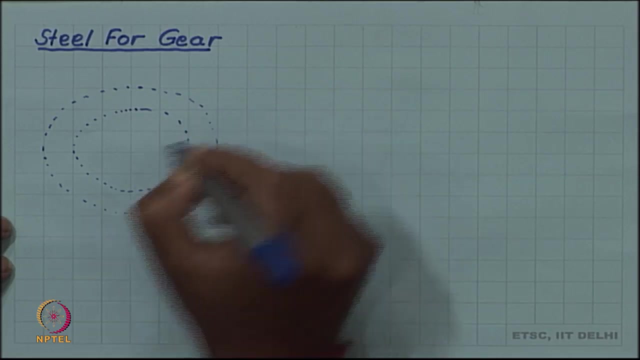 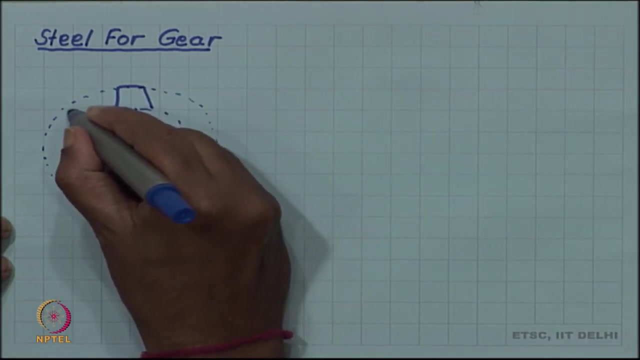 draw one for you. So I am trying to draw a gear which has teeth. So let us see. So I am trying to draw a gear which has teeth. So I am trying to draw a gear which has teeth. So 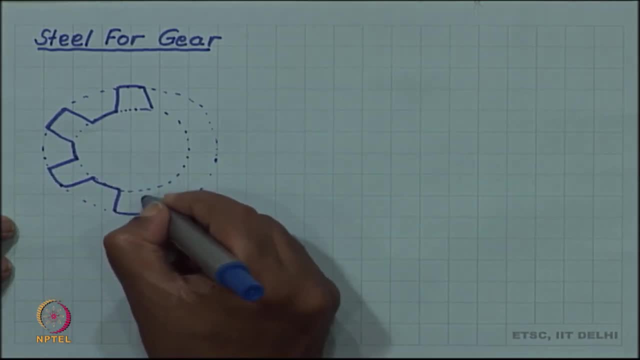 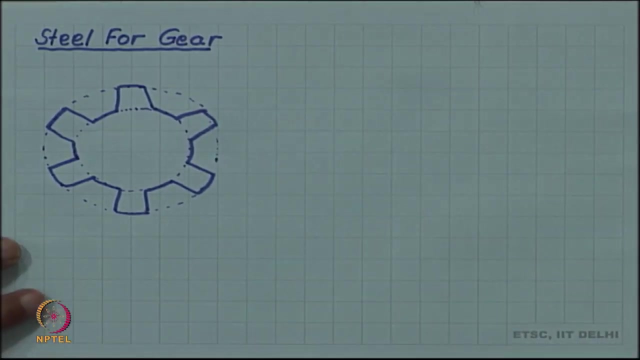 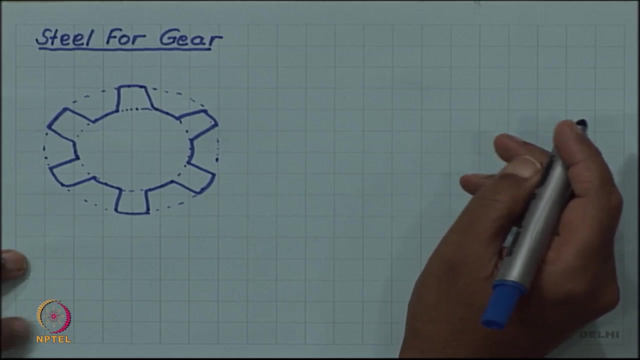 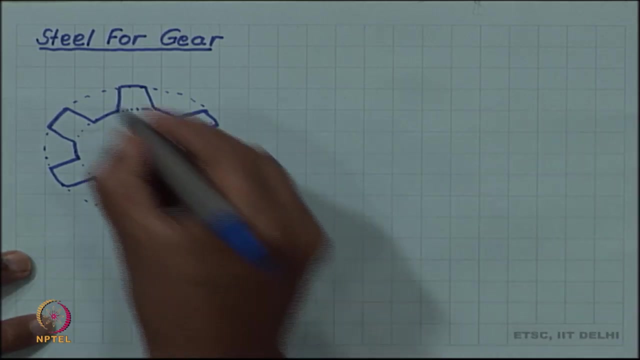 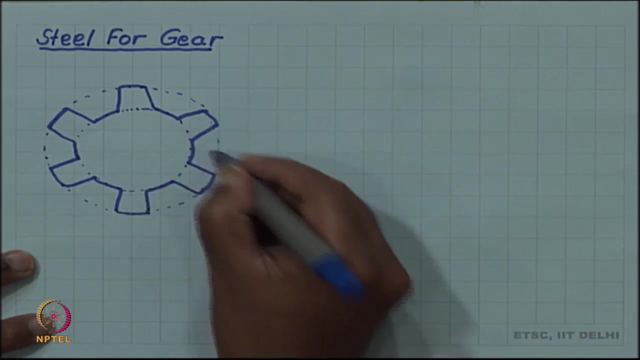 So- and this is gears, of course, are can be made of many materials. steel is a one common material of which gears are usually made in engineering. and what kind of steel should be select for this gear? Now, one thing: you can see very clearly that a gear messes with the teeth of other gear. 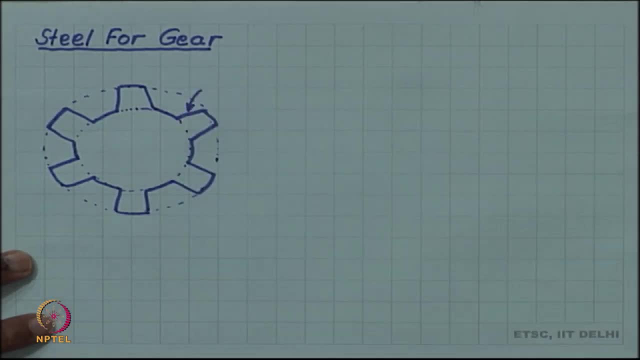 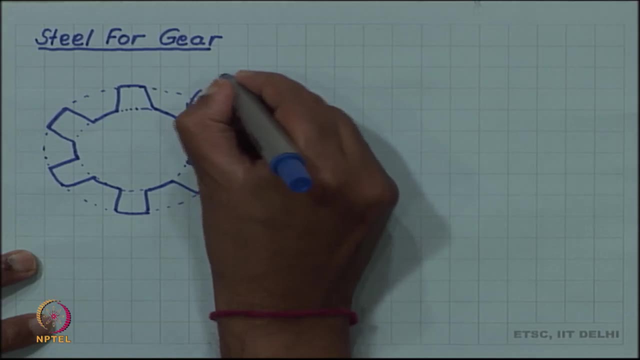 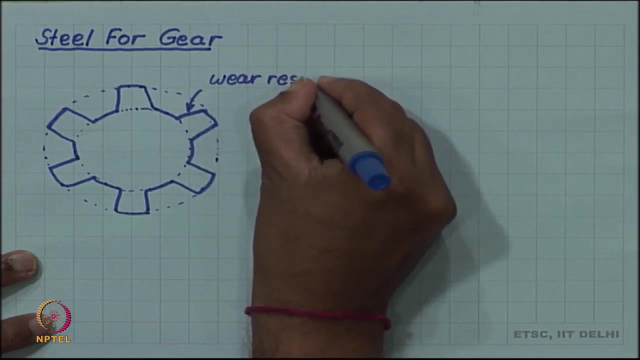 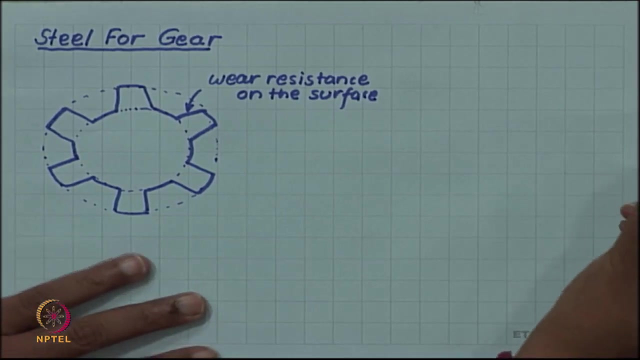 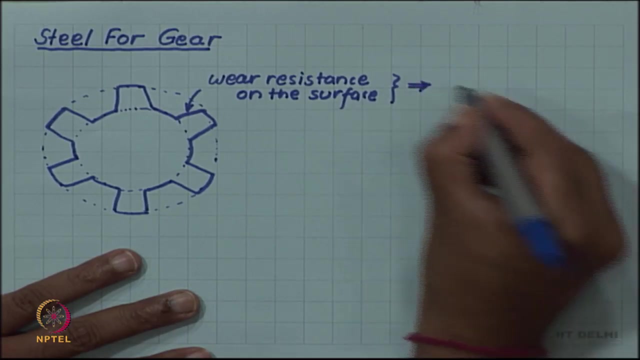 so there is lot of wear and rubbing on the teeth faces, so these faces should be wear resistant. So wear resistance is one of the requirement. now wear resistance requires harder the steel. higher is the hardness, higher is the wear resistance. So this imply that we should choose a steel of higher hardness and we have looked at 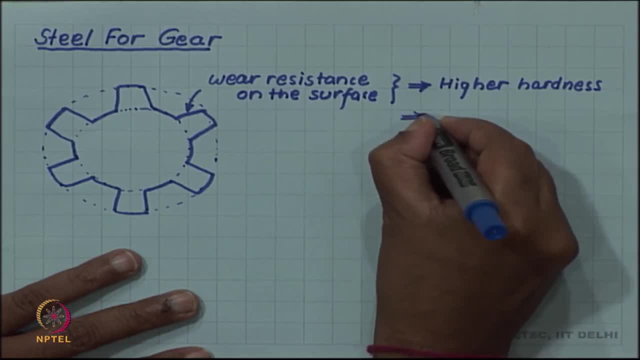 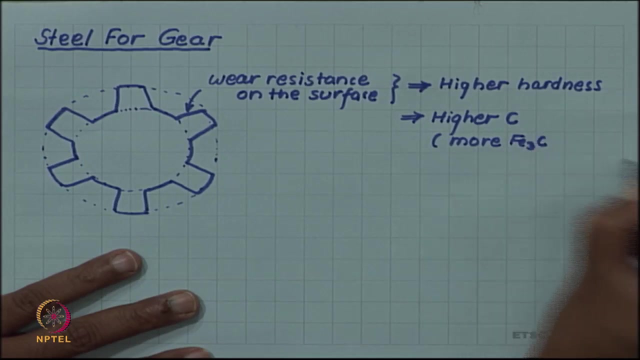 in the phase diagram that higher hardness comes from higher carbon. so we should select higher carbon steel, because higher carbon steel will have more Fe 3 C, for example, and this will increase, Increase hardness. so quite often higher hardness can be achieved by higher carbon. but we also 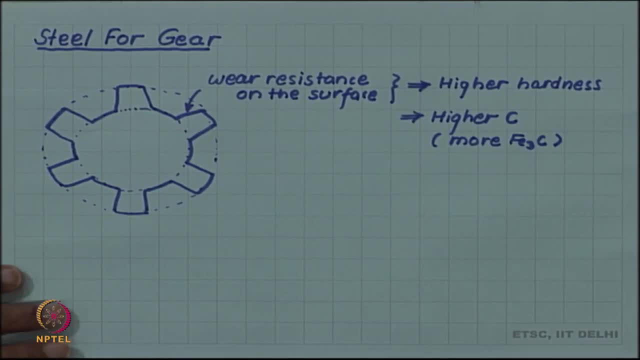 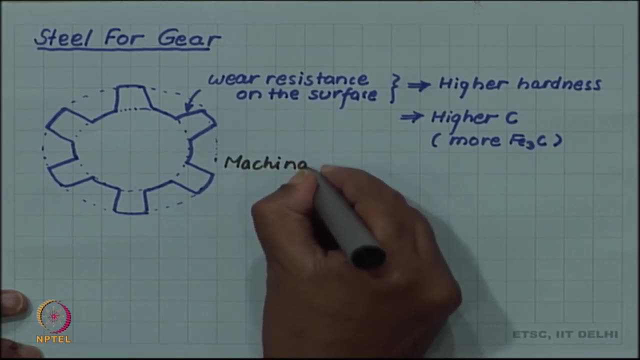 because we want to machine the gear in the forming process. we require machinability. 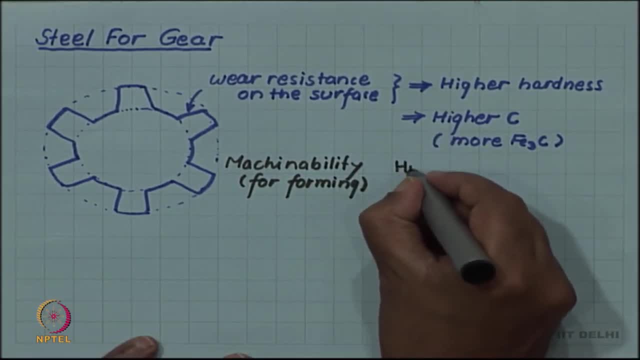 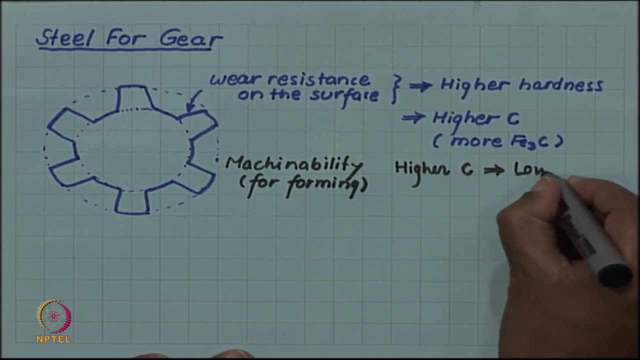 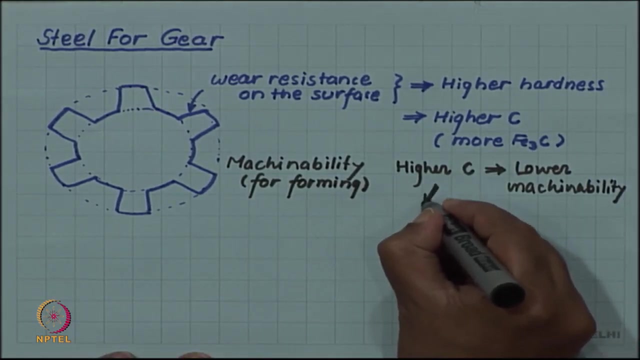 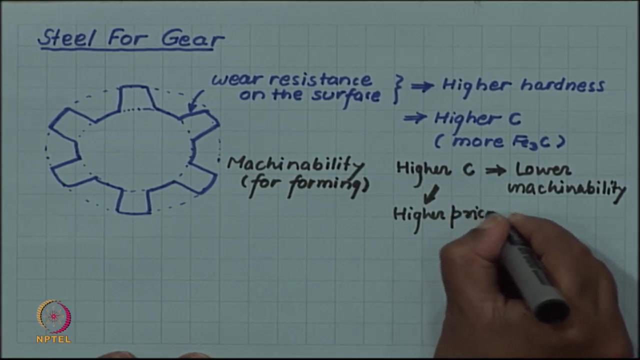 But machinability goes down with higher carbon. higher carbon implies lower machinability and also higher carbon also implies higher cost. So both the cost of the steel as well as the cost of processing will increase, higher the carbon we choose. 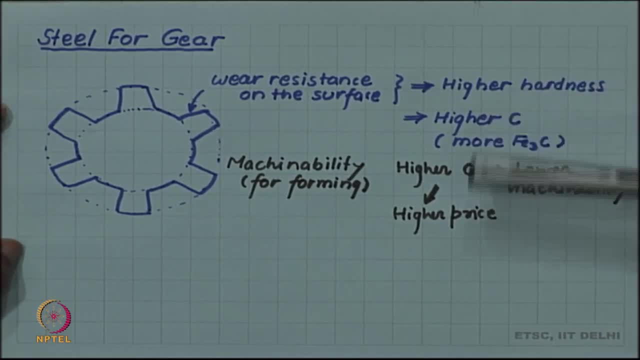 So you can see that there are two contradictory or two opposing requirements are there that of wear resistance, which tells us to choose a higher carbon steel, and that of machinability, which indicates that we should go for low machinability, as well as price, which tells 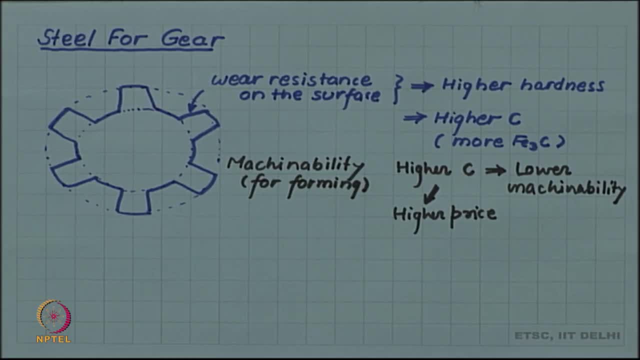 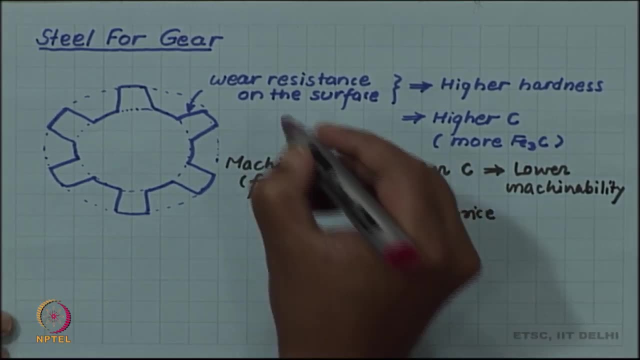 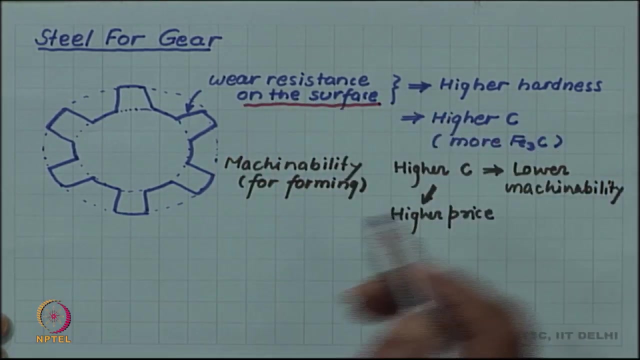 us that we should go for lower carbon concentrations. Now, optimization can be done if we note that wear resistance is required only on the surface, So we do not have to select a high carbon steel for the entire gear. The higher carbon concentration is only required. 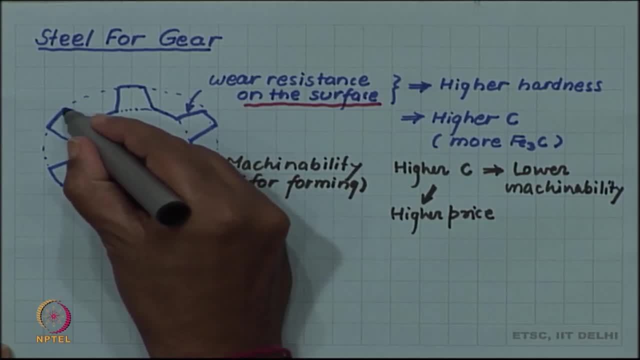 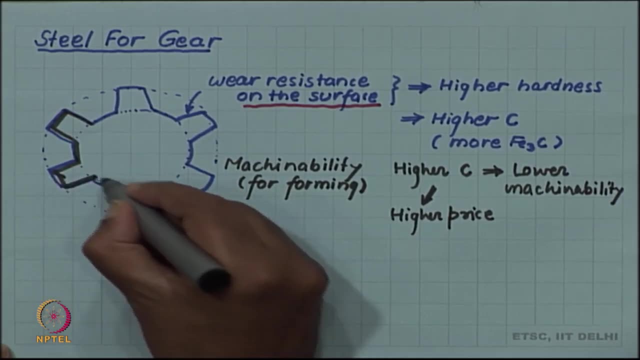 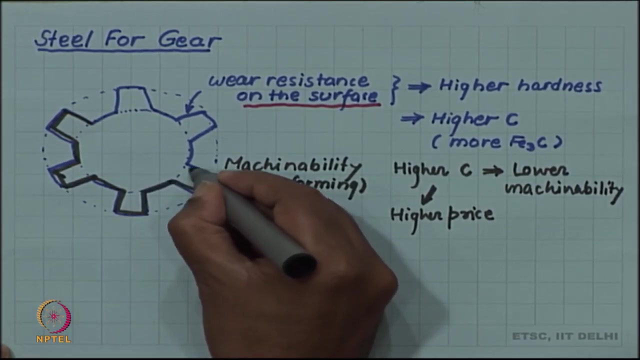 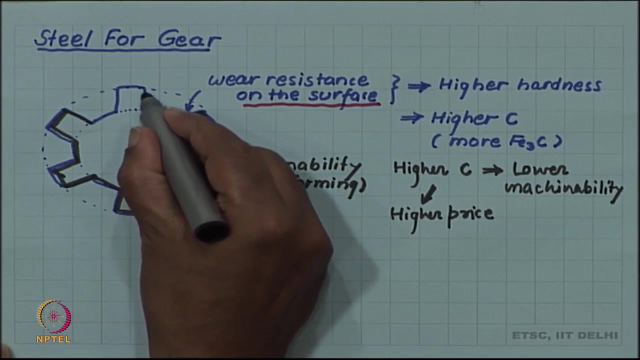 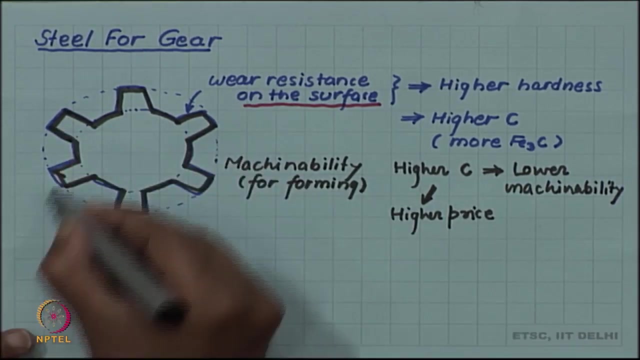 So if somehow we can make surface of higher carbon, then the wear resistance property will be satisfied. We need not make the entire steel of a high carbon. Is this possible? The question: is this possible? and it turns out that, yes, there is an engineering process. 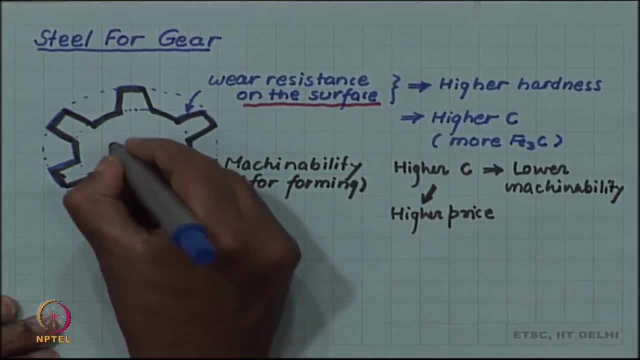 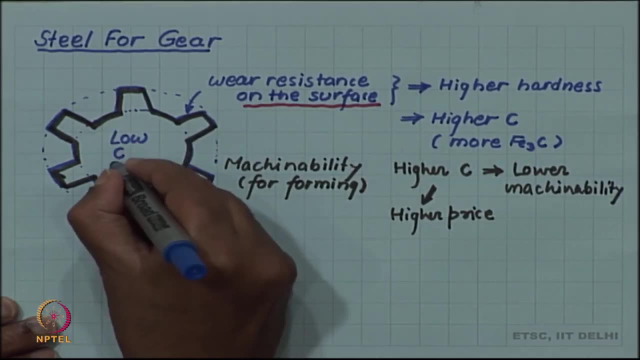 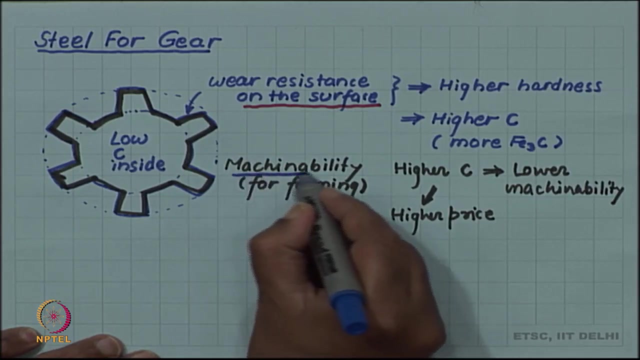 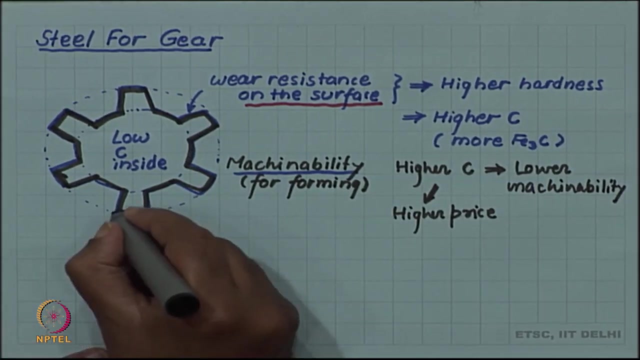 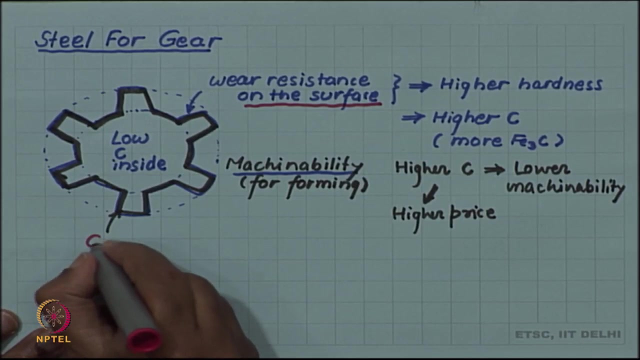 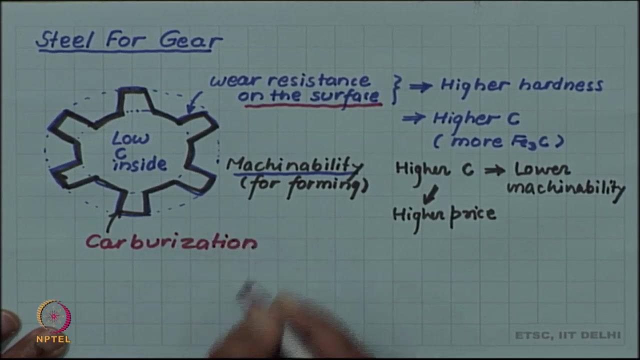 whereas we can start with a low carbon steel, So lower carbon in the interior, so we can start with low carbon steel. So this gives us good machinability. we can shape our gear and after shaping the gear, we can by a process called carburization. we have a process called carburization by 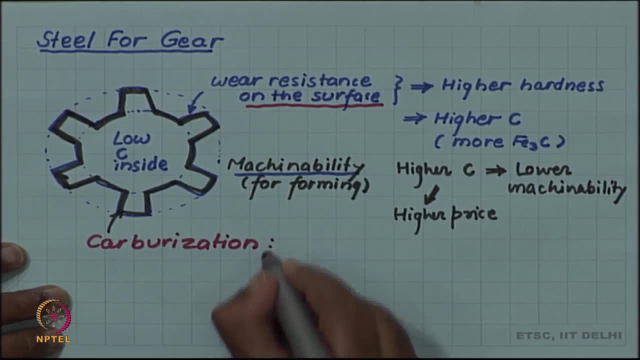 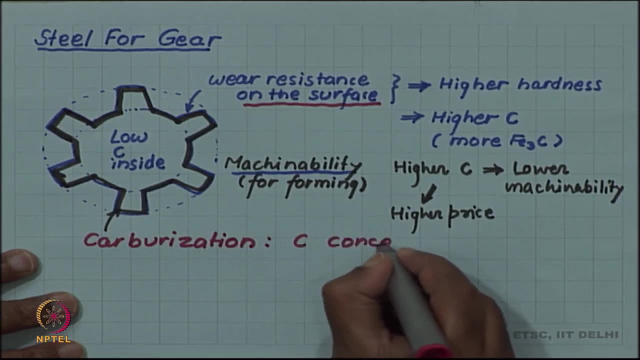 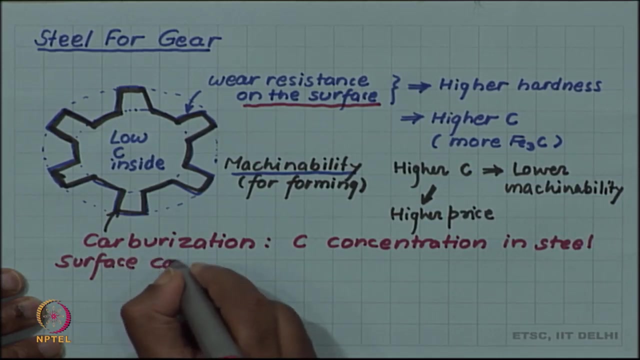 which the surface concentration of carbon can be changed or increased in the steel carbon concentration. So this is called carburization. So this is called carburization. So this is called carburization. So that is the process. 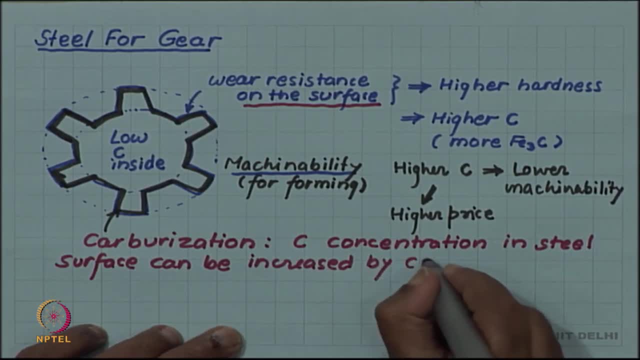 So this is the combustible environment where carbon is focused. This is called carburization. So the process is this: combination of rakin电etes and steel at one point, or rather a by carburization treatment. essentially, what you do in carburization is to heat the low. 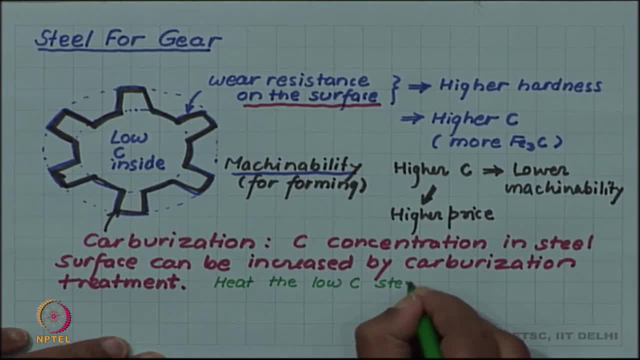 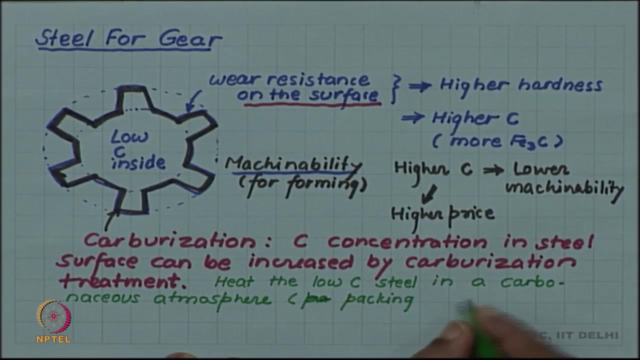 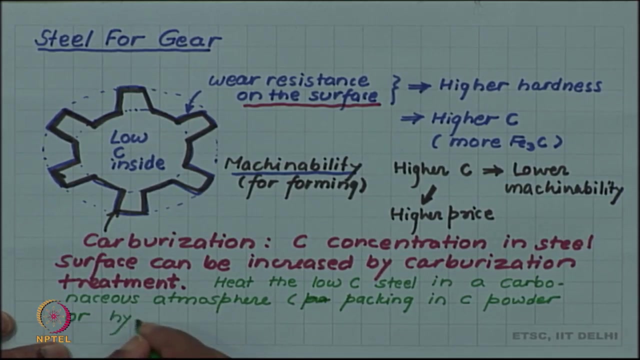 carbon steel in a carbonaceous atmosphere. So let us say we can achieve this by packing in carbon Carbon powder or we can use in gaseous atmosphere hydrocarbon gases, if you are doing a packing in carbonaceous powder. 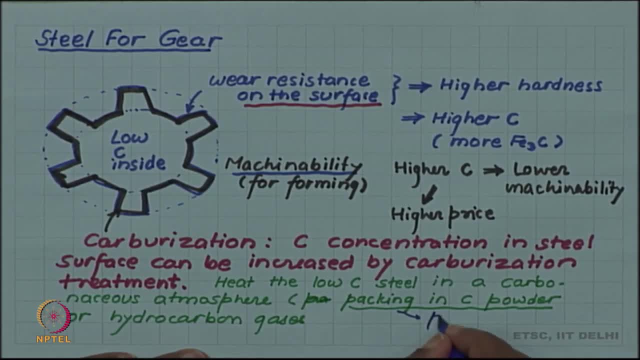 So there is a process of this is sometimes called pack carburization, and if you are using hydrocarbon gases, this is called gas carburization. You will not going into the details of carburization- heat treatment- here, but it is a what we want to emphasize, that 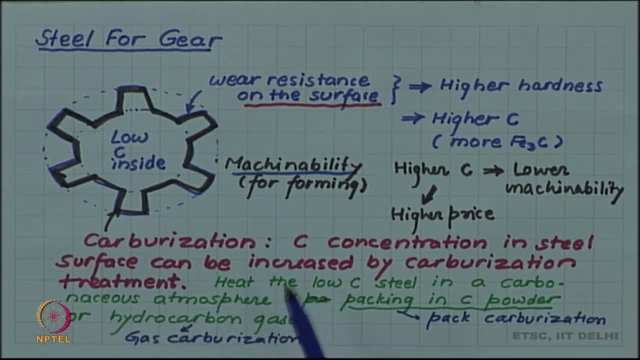 there is a process, engineering process available to us where we can start with a low carbon steel which has good machinability, So we can shape our gears easily and then- but such a gear will not have good wear resistance because it is of low carbon steel. Then we can improve. 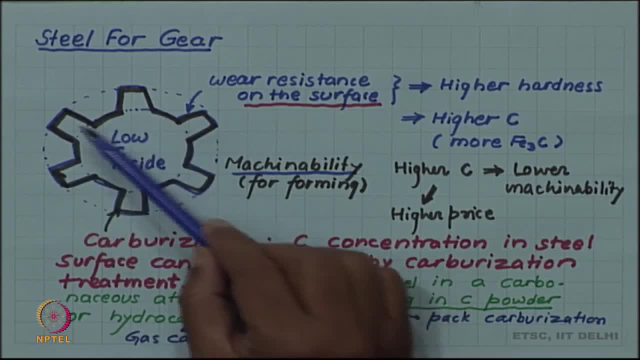 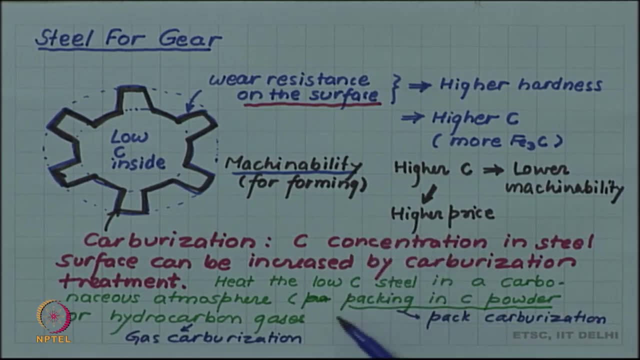 the wear resistance by increasing the carbon concentration on the surface by a process called carburization. But how does carbon from the atmosphere, from outside atmosphere, get into the steel? and that is the process of diffusion. So diffusion is required for carbon to enter into the steel and enrich the surface layer, So carburization is possible. 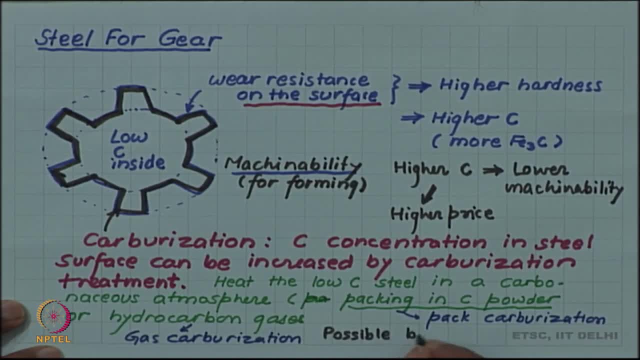 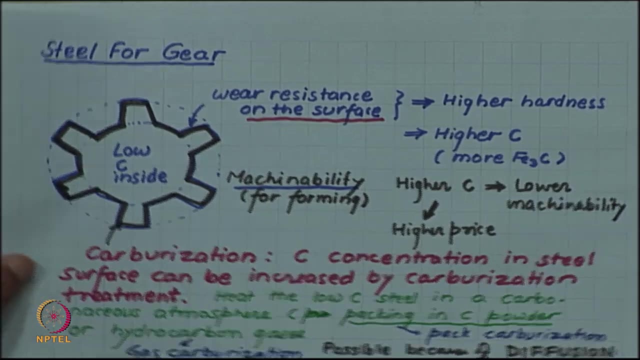 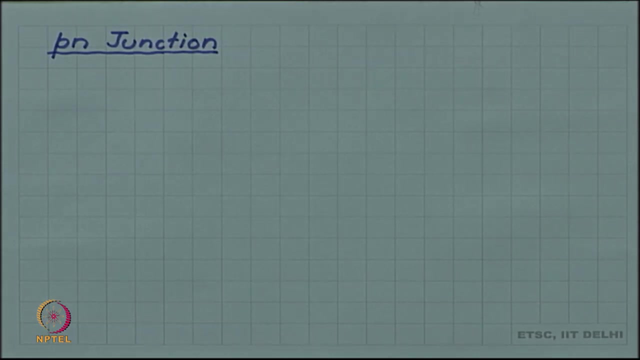 this is possible because of diffusion. Okay, Okay, Let us look at. this is a very classic example. let us look at little bit more recent, modern example, and that is forming of a p n junction When, for electronic circuits, a p n junction. 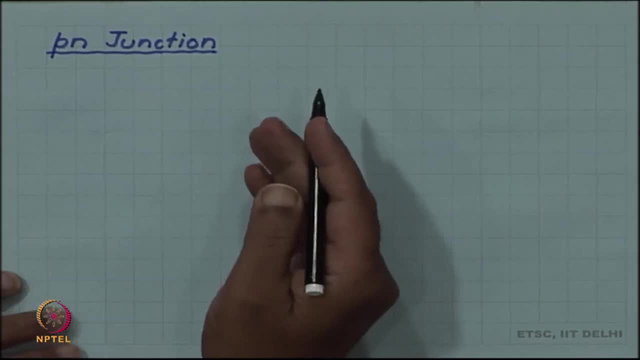 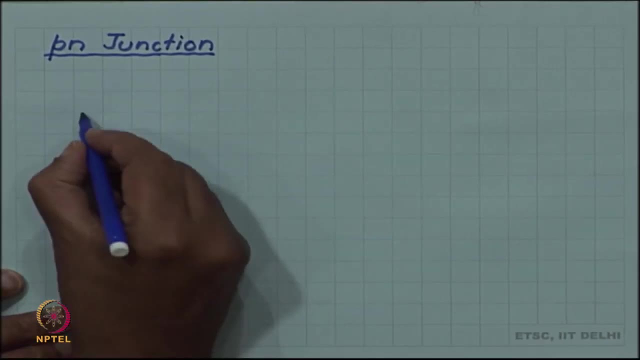 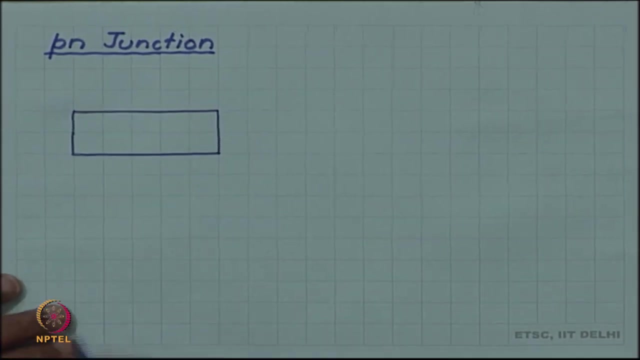 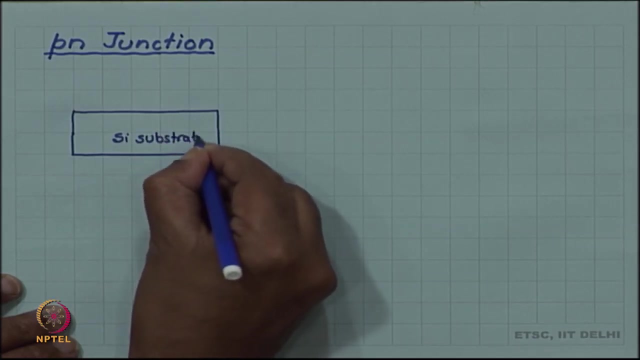 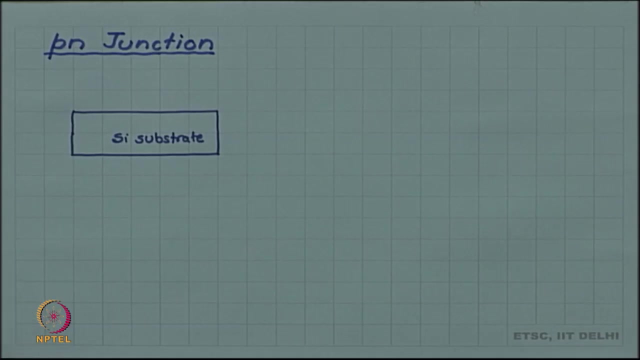 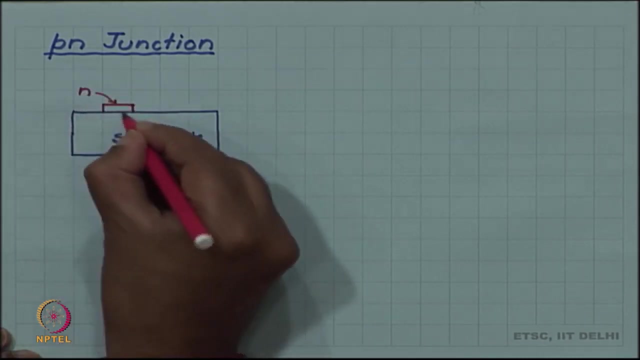 is formed. it is not formed by welding together a p type and an n type semiconductor. What is usually done Is that you have a, you have a silicon substrate and then you will deposit on it an n type region. Various deposition techniques are there, by which, let us say, this is n type and we